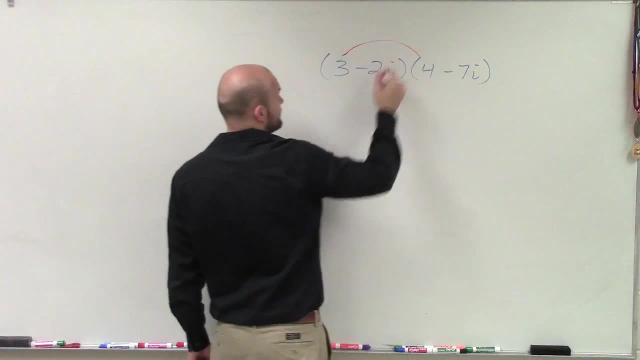 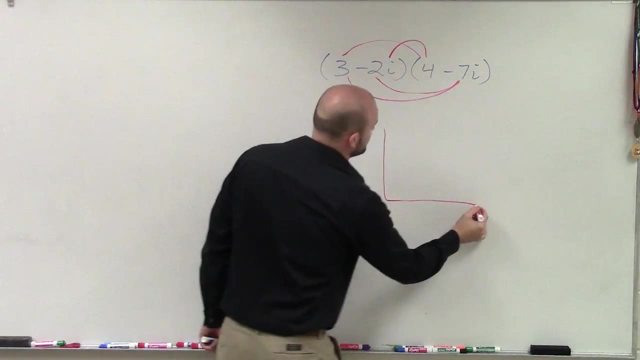 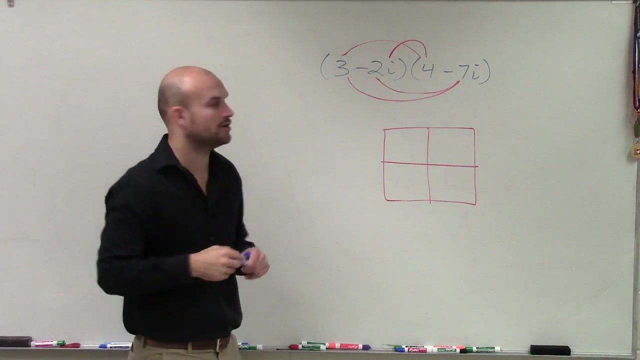 So, on the box method, all I'm simply doing, I'm doing FOIL, I'm doing the first, the outer, the inner and the last. But with the box method, all I simply do is I just write one binomial on top and one binomial on the side: 3 minus 2i, 4 minus 7i. 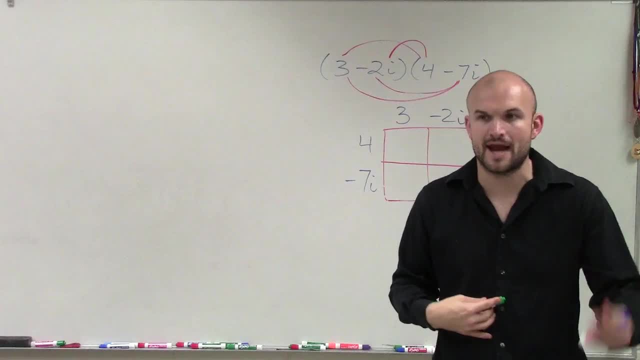 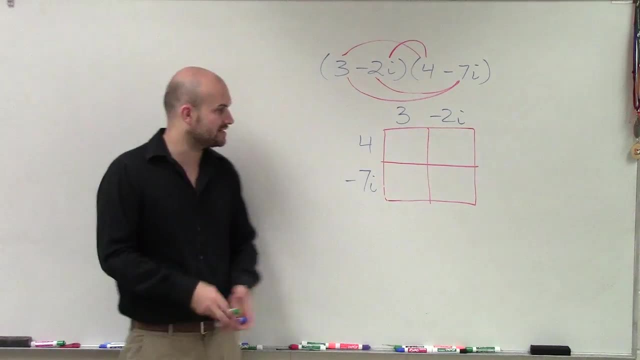 And because when we talk about multiplication, multiplication is finding the area of a figure, Even though this looks like pretty weird areas that we're talking about, because we're talking about a bunch of numbers, but that's what multiplication is. So what I do is now I just take each rectangle and I find the area. Remember, 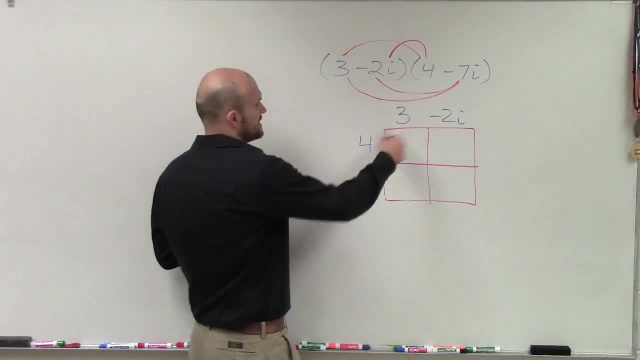 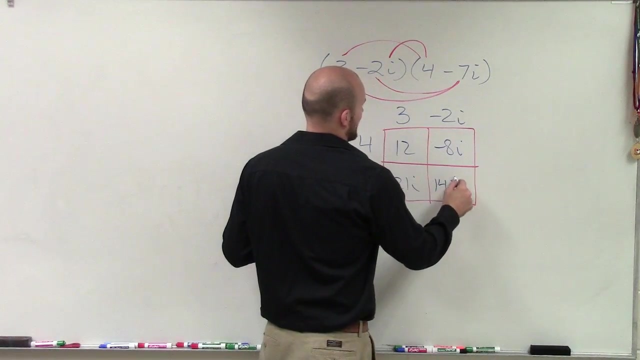 finding the area would just be length times width. So I do 3 times 4,, which is 12.. 4 times negative 2 is negative 8i. 3 times negative 7i is a negative 21i, And then negative 7i times negative 2i is going to be a positive 14i squared. 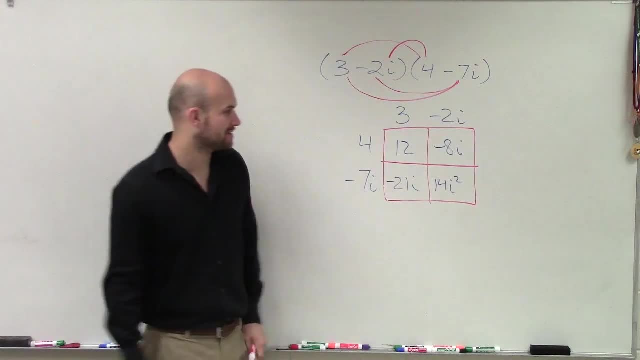 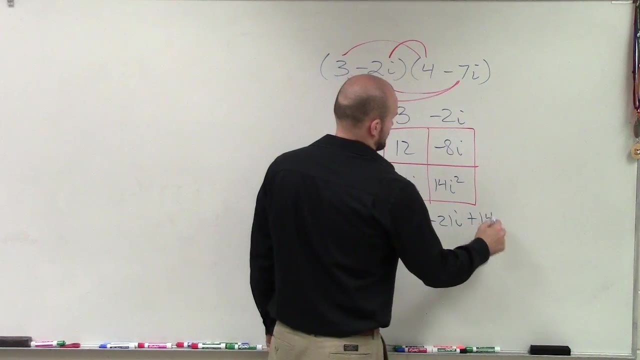 Now you can simplify from in the box, But I'm going to write it out just to make sure nobody's making the same mistakes in the other boxes. OK, Now remember, I told you guys 14i squared. Yes, you can do the i's and the dot's. 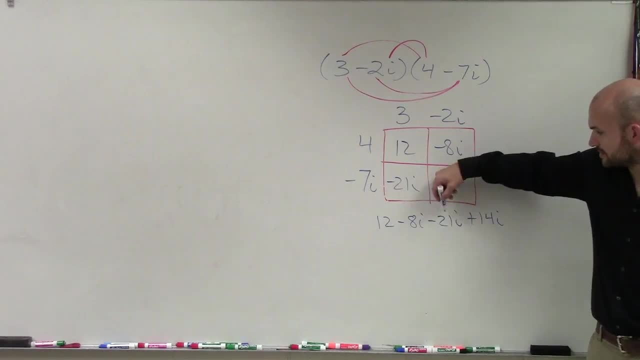 Remember I told you guys think of these as polynomials. You can combine these middle terms. These both have i, so it's the same imaginary factor, So you can combine them. yes, 14i squared, Thank you, So I can combine these. 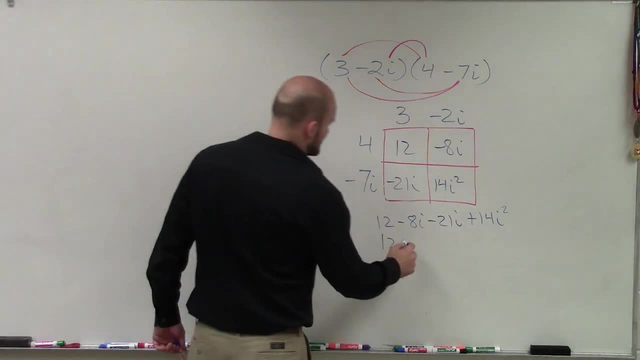 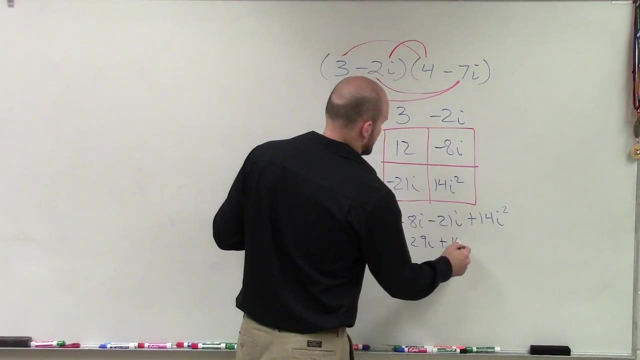 So I can combine these into 12.. Negative 8 minus 21i is a negative 29i. And then I have 14i squared. Well, remember, 14i squared is 14 times i squared, which is a negative 1.. 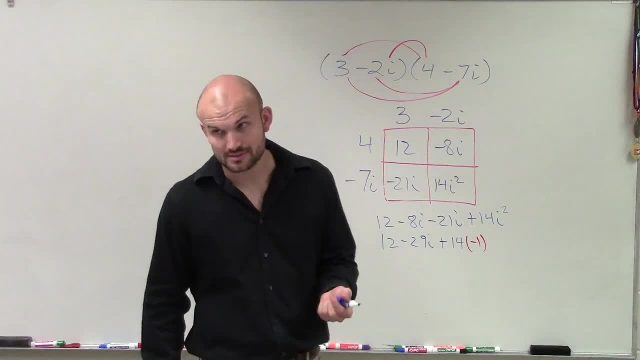 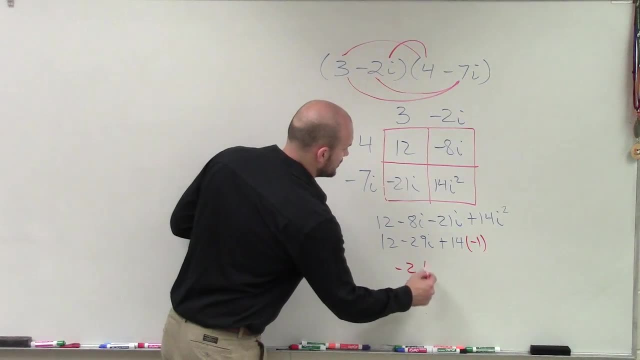 You have to remember that i squared is negative 1. It gets a lot of students, A lot of students. So now I have negative 14 and I have a positive 12.. So my final answer is negative 2 plus- I'm sorry, negative 2 minus 29.. 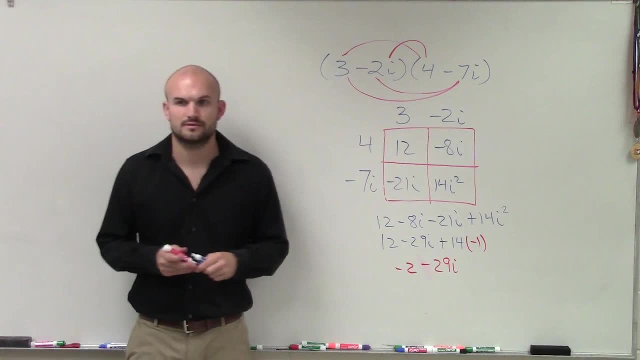 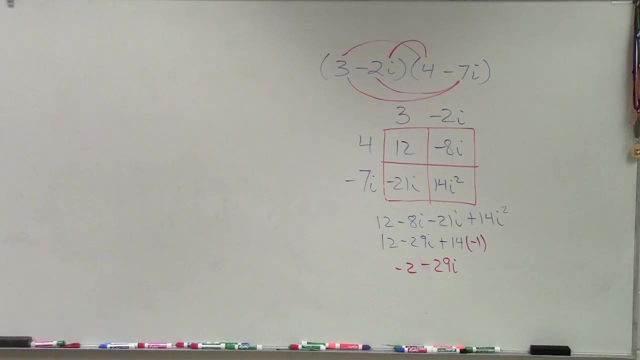 I And that's your final answer. OK, Cool, Good stuff, I guess. Good talk, All right, Thank you. Good, Let's do one last problem. I forgot to do one of these.